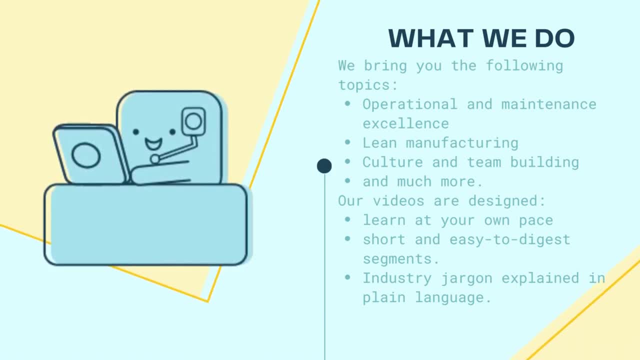 Our videos are designed with you in mind. Learn at your own pace with short and easy-to-digest segments, And don't worry about industry jargon. We use it when needed, but we also explain each section in plain language, So sit back, relax. 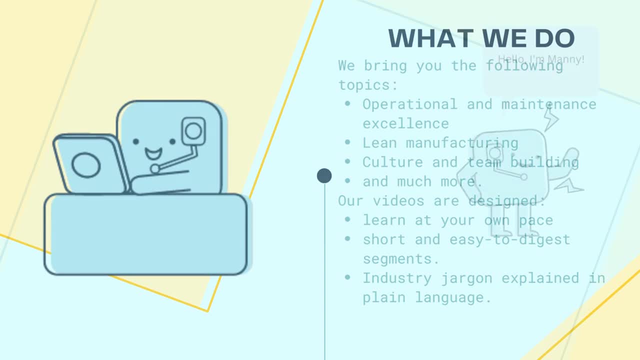 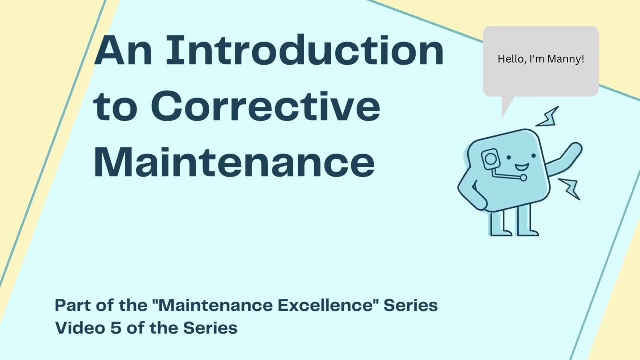 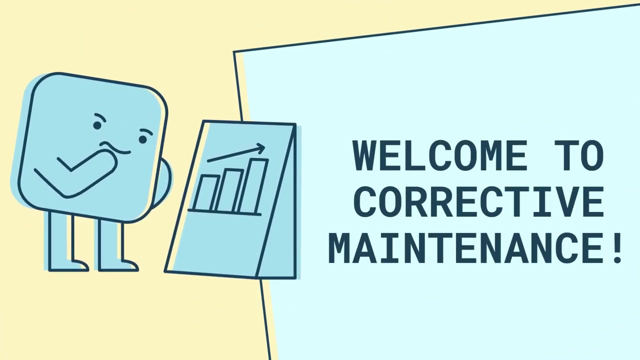 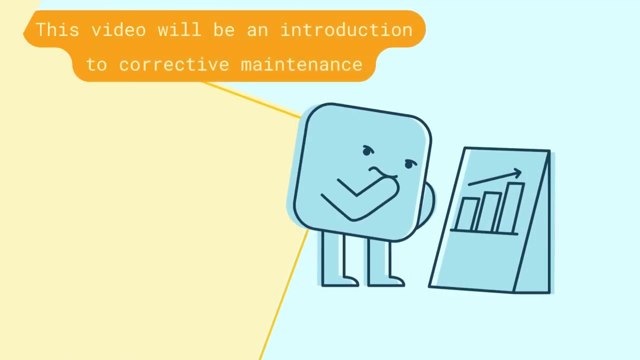 And let's dive into the world of manufacturing together. Hello, I'm Manufacturing, Manny. I will be your guide as we explore an introduction to corrective maintenance. This is part 5 of the Maintenance Excellence series. Welcome to our educational video on corrective maintenance, where we dive into the world of maintenance strategies and explore how they contribute to operational excellence. 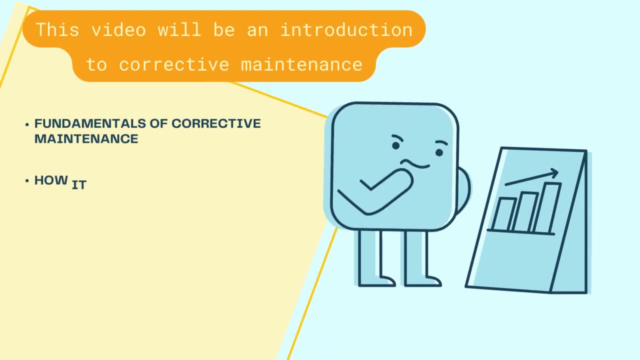 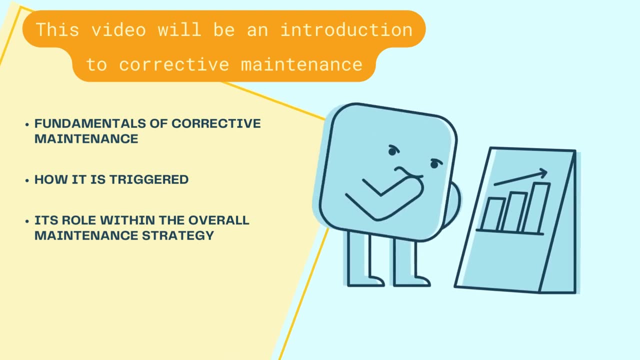 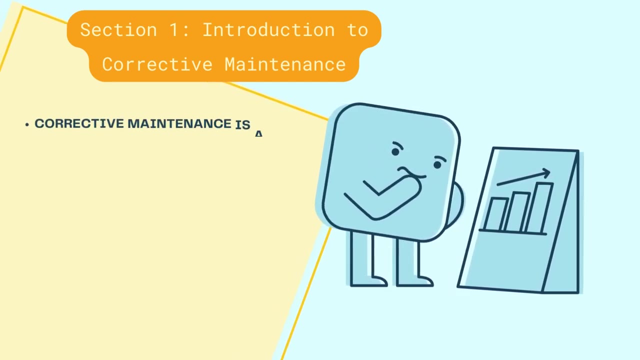 In this video, we'll cover the fundamentals of corrective maintenance, Its triggers and its role within the overall maintenance strategy. So let's get started. Section 1: Introduction to Corrective Maintenance. Corrective maintenance is a crucial aspect of maintaining equipment reliability and minimizing disruptions. 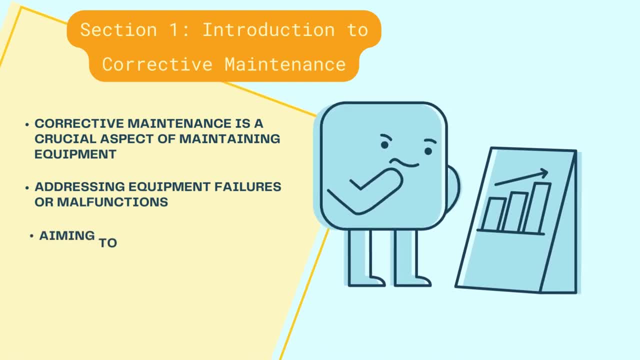 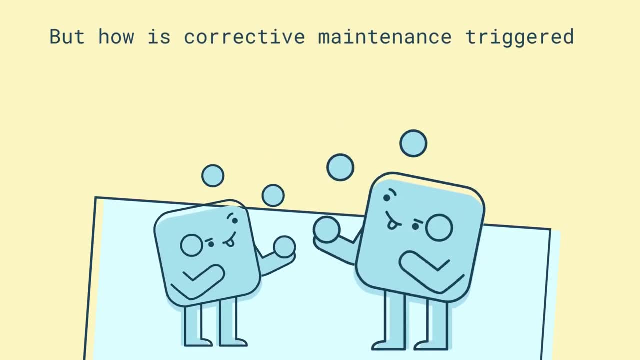 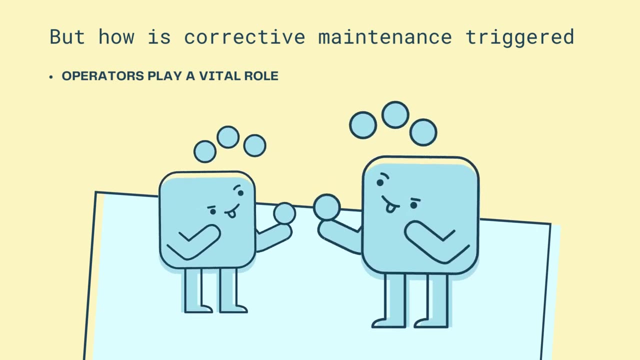 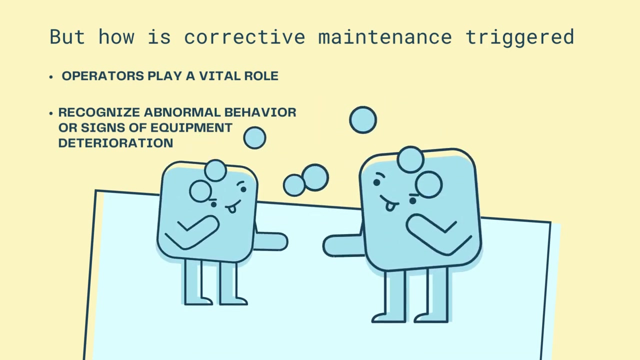 It involves addressing equipment failures or malfunctions, aiming to restore normal operation. But how is corrective maintenance triggered? Corrective maintenance can be triggered by various factors. Operators play a vital role in identifying issues during their daily operations. Their knowledge and experience allow them to recognize abnormal behavior or signs of equipment deterioration. 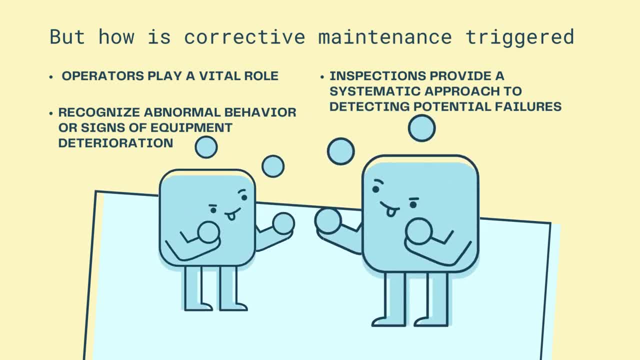 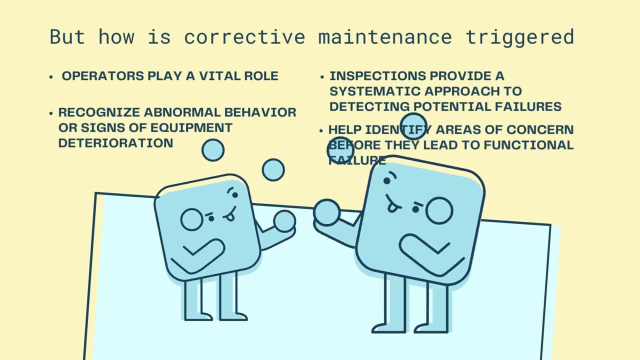 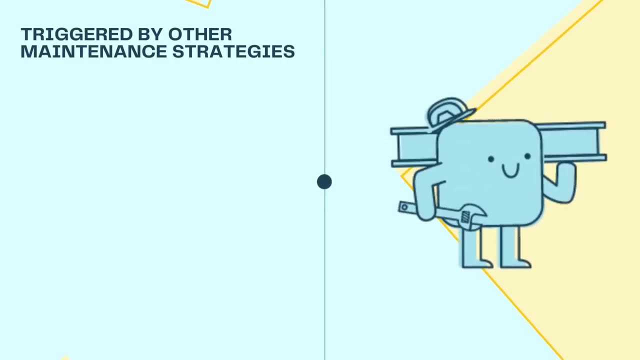 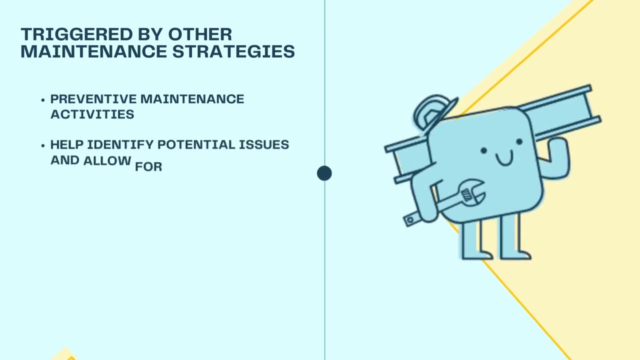 Additionally, inspections provide a systematic approach to detecting potential failures. Regular inspections and condition assessments help identify areas of concern before they lead to functional failure. Standard maintenance- Corrective maintenance- can also be triggered by other maintenance strategies. Preventive maintenance activities, such as routine inspections and scheduled replacements, help identify potential issues and allow for timely corrective action. 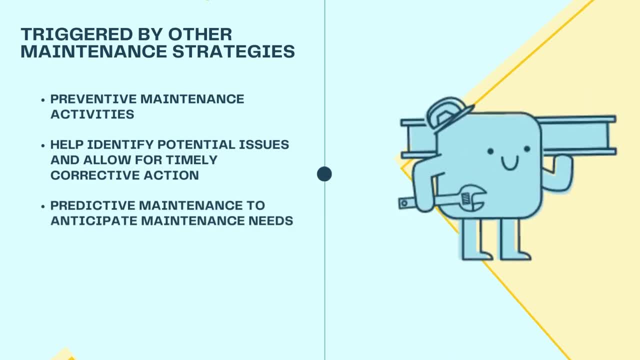 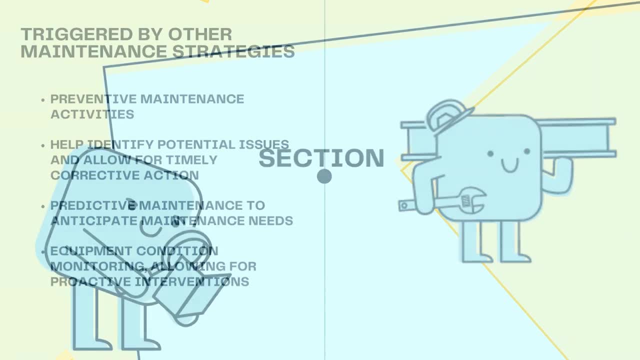 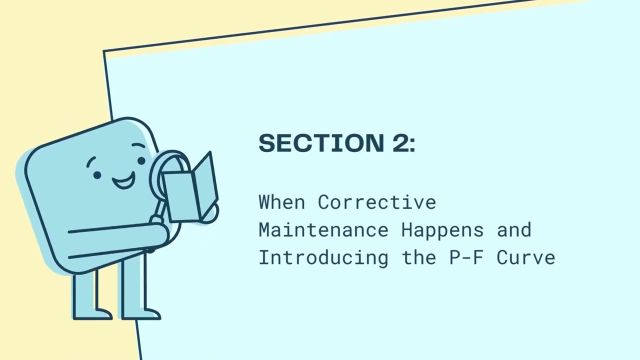 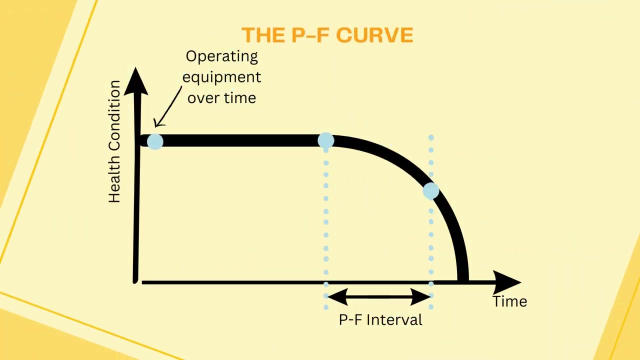 Similarly, predictive maintenance leverages data and analytics to anticipate maintenance needs based on equipment condition monitoring, allowing for proactive interventions. Section 2: When corrective maintenance happens, maintenance happens and introducing the PF curve. To better understand how corrective maintenance is triggered, let's introduce the PF curve. The PF curve is a valuable tool for understanding. 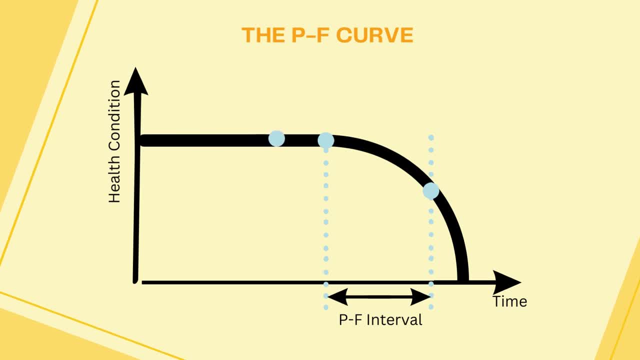 equipment failures and their progression. It consists of two key points: the potential failure P and the functional failure F. The potential failure P represents the point at which a component shows signs of degradation, indicating that a failure is imminent. It serves as a trigger. 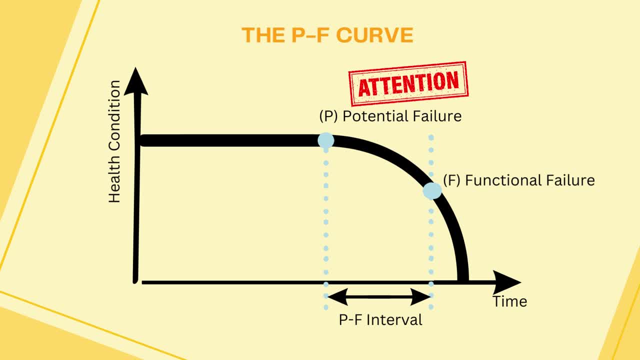 for corrective maintenance. By identifying the potential failure point through condition monitoring or other indicators, maintenance teams can intervene and prevent the equipment from reaching the functional failure F stage. Corrective maintenance triggered by the PF curve can be associated with different maintenance strategies. Reactive maintenance occurs when: 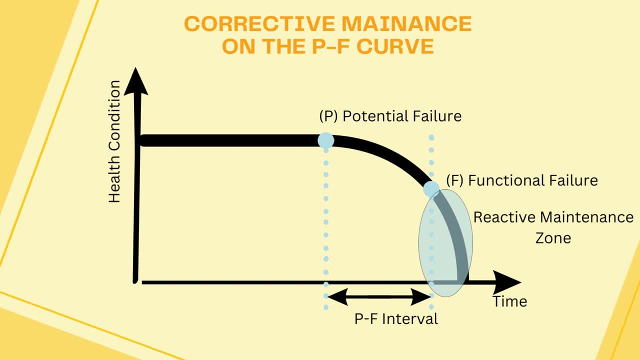 failures are addressed only after the failure is committed. The PF curve is a tool for understanding the potential failure P in a diferentes area. Preventive maintenance involves scheduled tasks performed at regular intervals to prevent failures, including actions triggered by the potential failure point on the PF curve. Predictive maintenance utilizes advanced analytics and. 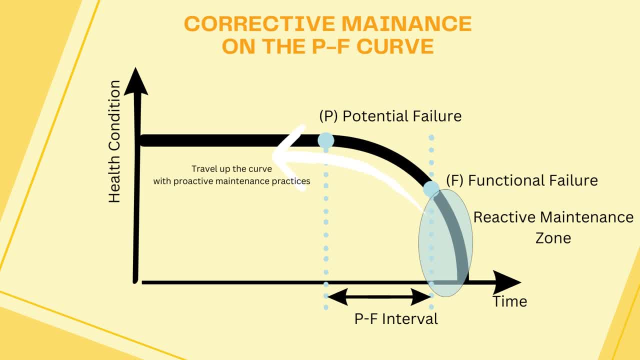 condition monitoring to predict maintenance needs and intervene before functional failure occurs. Finally, condition-based maintenance focuses on performing maintenance tasks based on specific maintenance challenges. Using P in the PF curve can ensure corrective maintenance, equipment conditions or indicators, including those identified through the potential failure. 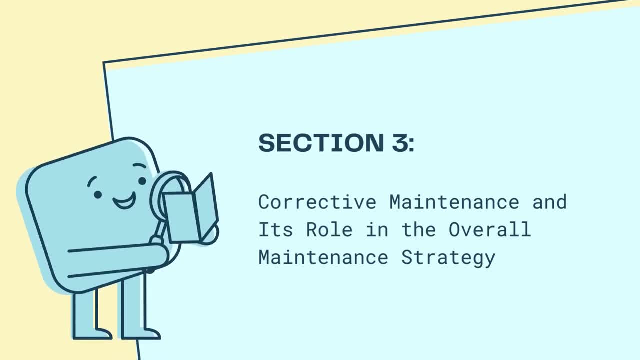 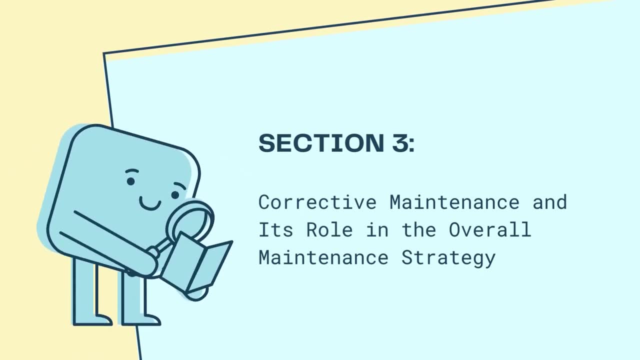 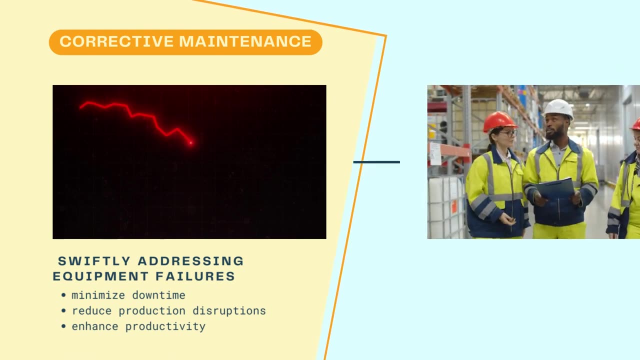 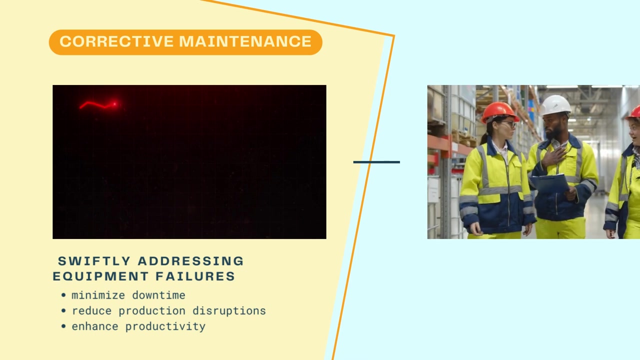 point Section 3. Corrective Maintenance and Its Role in the Overall Maintenance Strategy. Corrective maintenance offers numerous benefits that contribute to operational excellence. By swiftly addressing equipment failures, organizations can minimize downtime, reduce production disruptions and, ultimately, enhance productivity When corrective maintenance is performed efficiently and effectively. 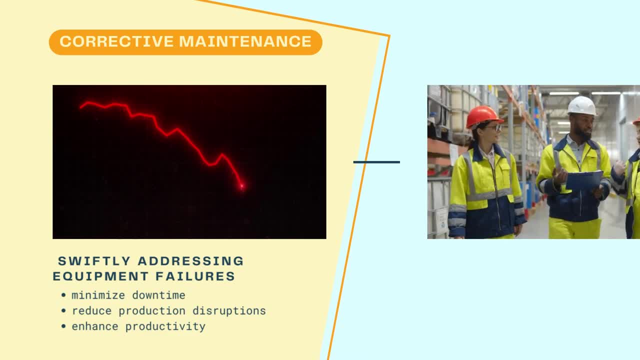 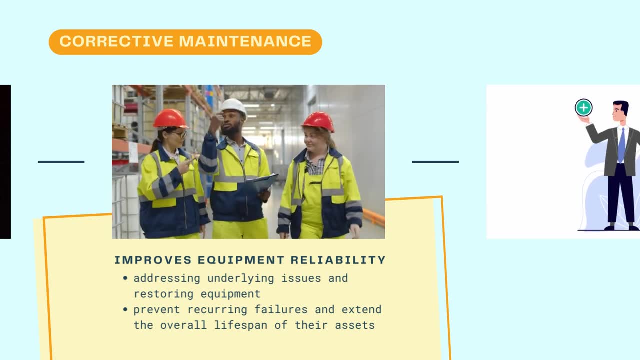 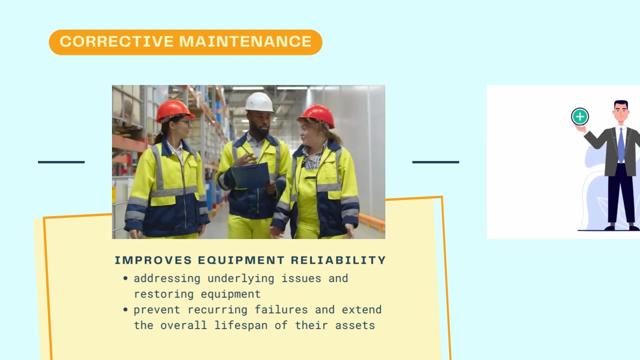 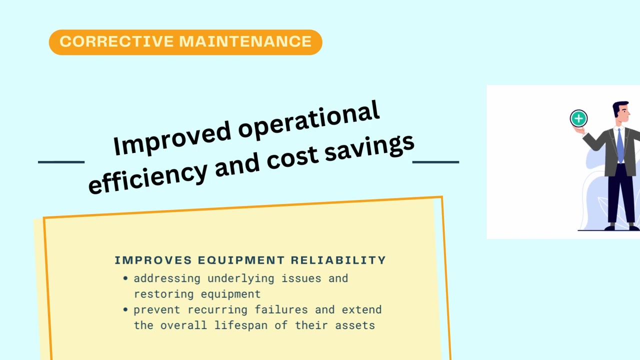 it helps maintain a smooth and uninterrupted workflow. In addition to reducing disruptions, corrective maintenance improves equipment reliability. By addressing underlying issues and restoring equipment to its optimal operating condition, organizations can prevent recurring failures and extend the overall lifespan of their assets. This, in turn, contributes to improved operational. 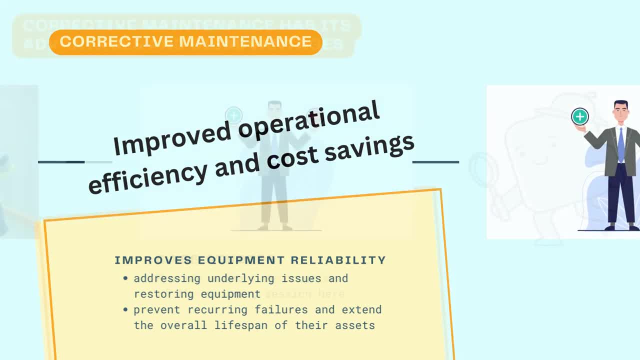 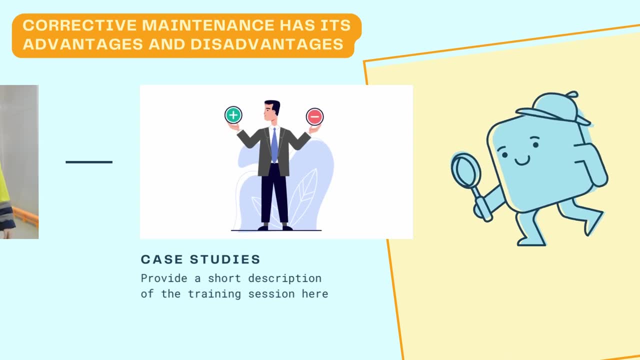 efficiency and efficiency of the organization. However, like any maintenance strategy, corrective maintenance has its advantages and disadvantages. On the positive side, corrective maintenance allows organizations to focus resources on addressing failures as they occur, making it a reactive approach. However, it can also lead to higher costs due to unplanned repairs. 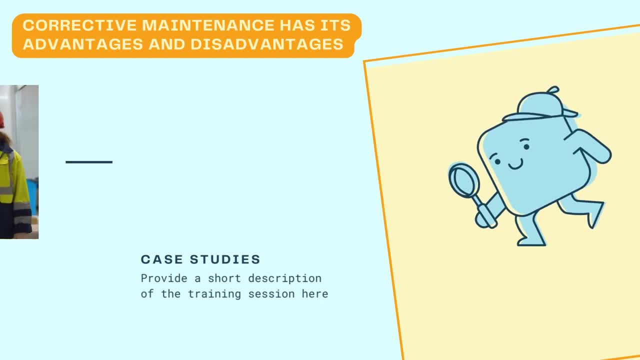 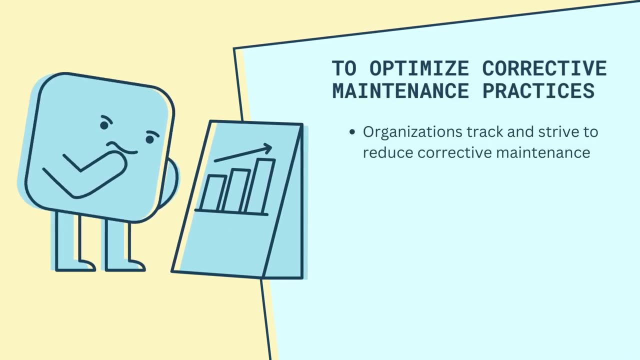 the need for replacement parts and potential production losses during equipment downtime? To answer this question, corrective maintenance is a great way to increase efficiency and cost savings. To optimize maintenance practices, organizations track and strive to reduce corrective maintenance through proactive measures such as implementing preventive. 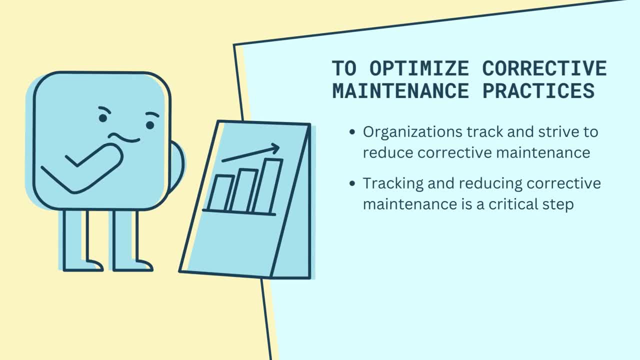 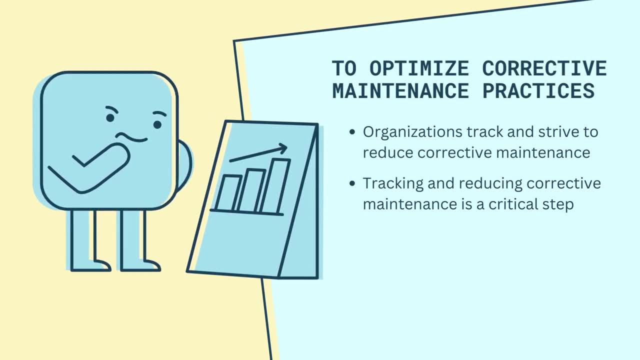 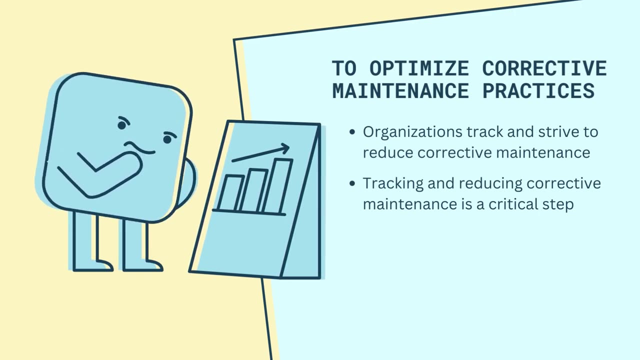 and predictive maintenance strategies. Tracking and reducing corrective maintenance is a critical step towards achieving maintenance excellence. By keeping records of corrective maintenance activities, organizations can analyze failure patterns, identify recurring issues and take proactive measures to address underlying causes. Root cause analysis plays a vital role in reducing corrective maintenance. 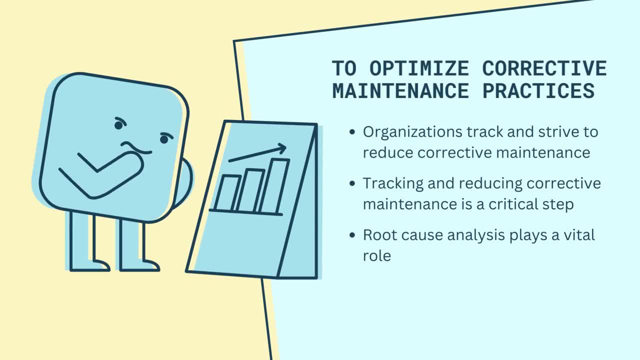 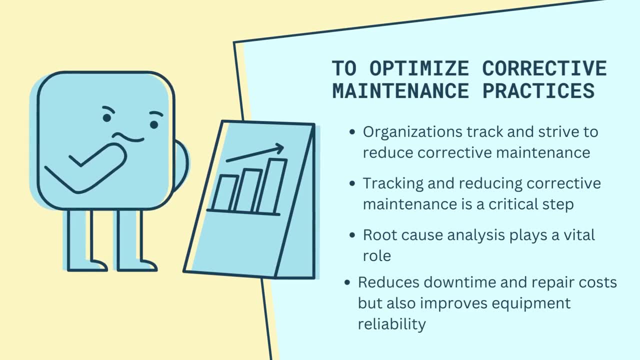 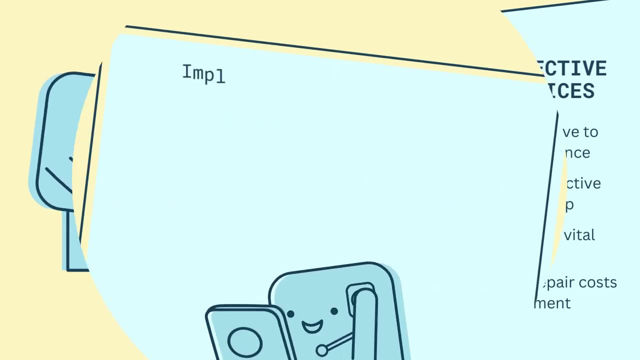 By identifying the root causes of failures, organizations can implement corrective actions that prevent similar issues from recurring. This approach not only reduces downtime and repair costs, but also improves equipment reliability and overall maintenance effectiveness. Implementing preventive and predictive maintenance strategies can also contribute to reducing corrective maintenance. 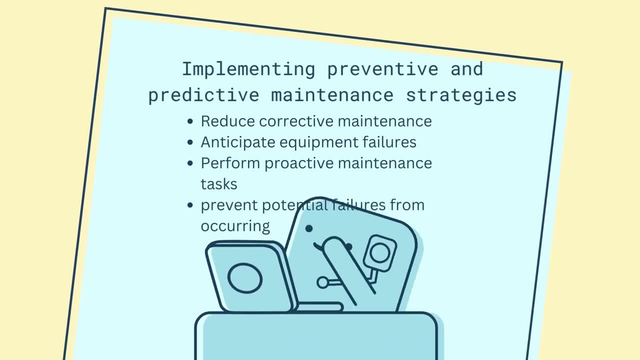 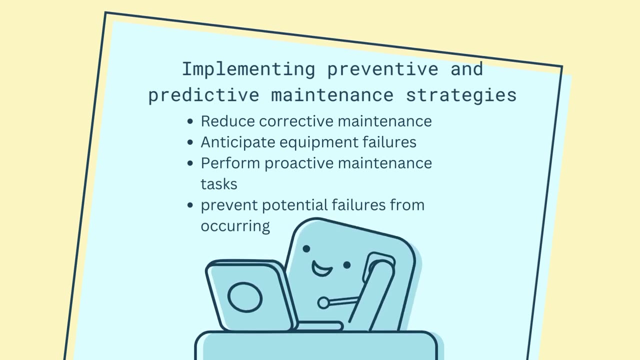 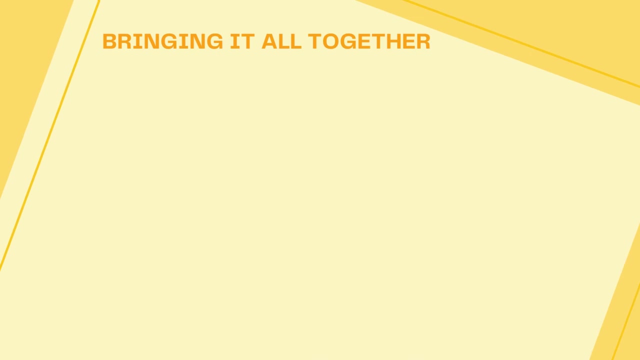 By leveraging data and analytics, organizations can anticipate equipment failures, perform proactive maintenance tasks and prevent potential failures from occurring. This shift towards proactive maintenance helps organizations minimize reactive maintenance and its associated costs and disruptions. Bringing it all together and summarizing: corrective maintenance: Corrective maintenance is an integral part of any maintenance strategy. 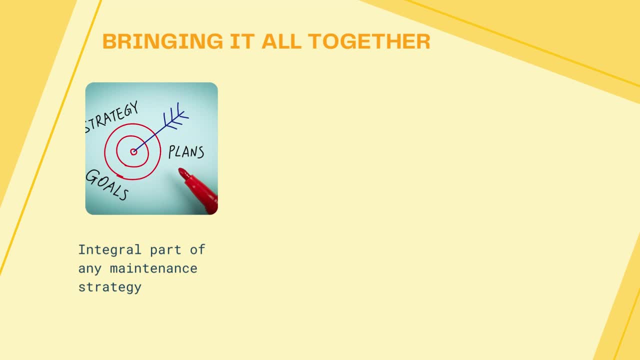 By promptly addressing equipment failures and malfunctions, organizations can maintain operational continuity, improve equipment reliability and optimize their maintenance processes. We explored the triggers of corrective maintenance, including operator observations, inspections and the role of preventive and predictive maintenance practices. We also discussed the PF curve and how it helps in understanding the progression of failures and 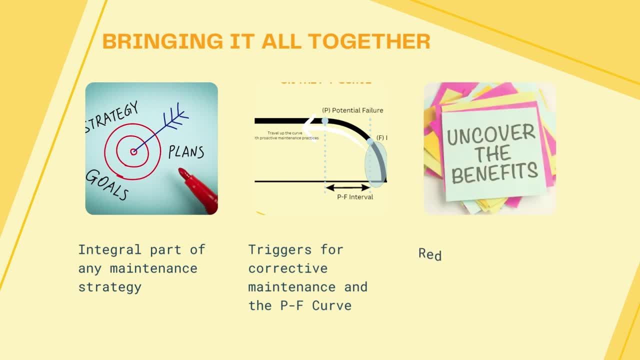 triggering corrective maintenance actions. We also discussed the PF curve and how it helps in understanding the progression of failures and triggering corrective maintenance actions. Additionally, we highlighted the benefits of corrective maintenance, such as reducing disruptions, improving equipment reliability and enhancing overall operational efficiency.